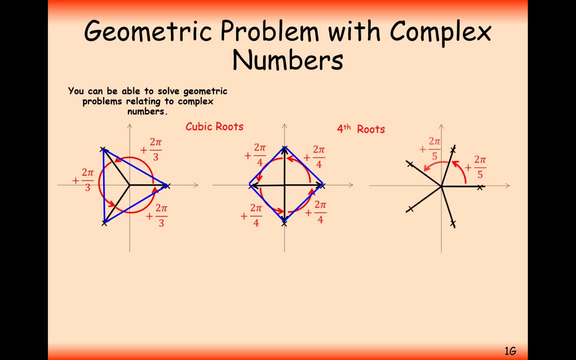 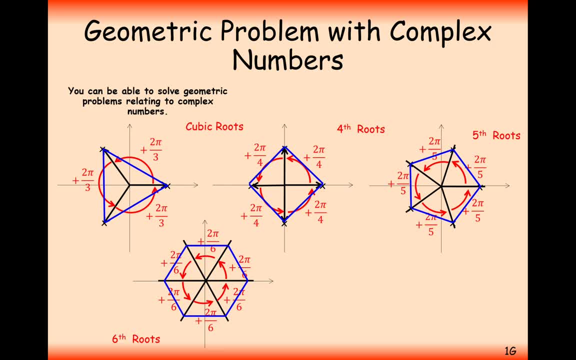 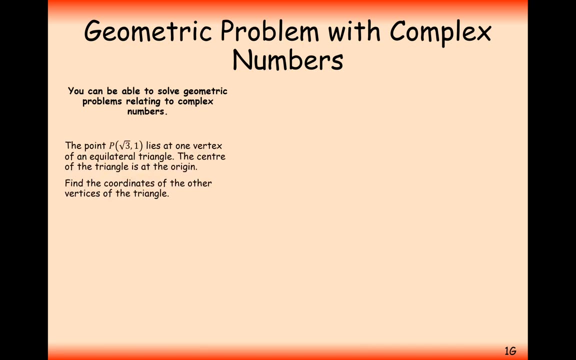 round the circle on the argument to get your perfect hexagon and then the last one here, the heptagon. just keep on adding 2 pi by 7 onto the argument and that will give you your perfect heptagon. So let's see a question in action. then The point root 3, 1 lies on. 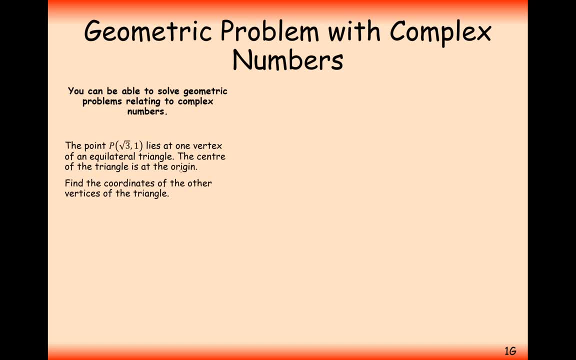 one vertex of an equilateral triangle. The centre of the triangle is at the origin. Find the coordinates of the other vertices of the triangle. So what we've effectively got is we've got root 3, 1 on the Argand diagram. So the first thing we're going to do to make 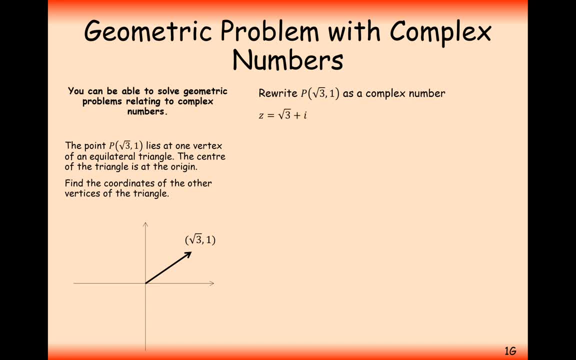 this into a complex number. problem is to write it as a complex number. Then we're going to write it in modulus argument form because that's easier to deal with when we're rotating it around the circle. Because to rotate it around the circle and make an equilateral 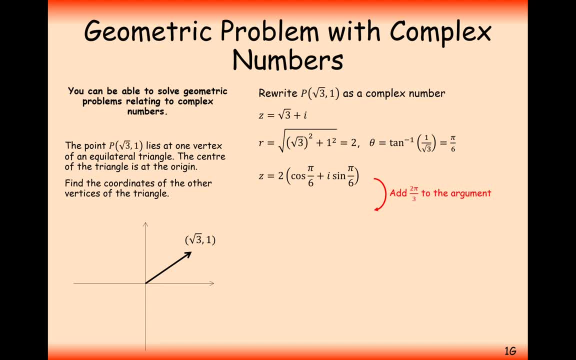 triangle. you just need to add 2 pi by 3 to the argument. Let's get to the next one. So that would be 5 pi by 6.. Add another 2 pi by 3 onto the argument and that will get you to 9 pi by 6, but that's outside of the range from minus. 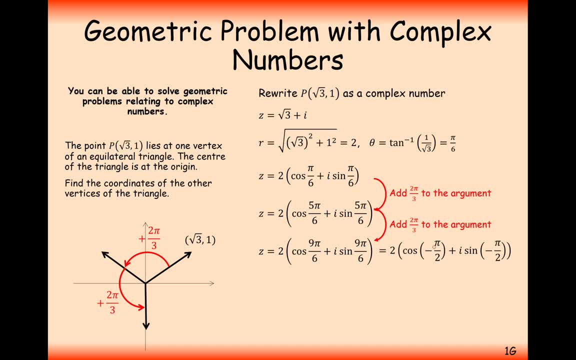 pi to pi- so we'll need to do a correction on that- to minus pi by 2.. So these are our three roots. then What we'll now need to do is expand the modulus argument form to get the Cartesian form of the complex numbers and then just rewrite the Cartesian form of. 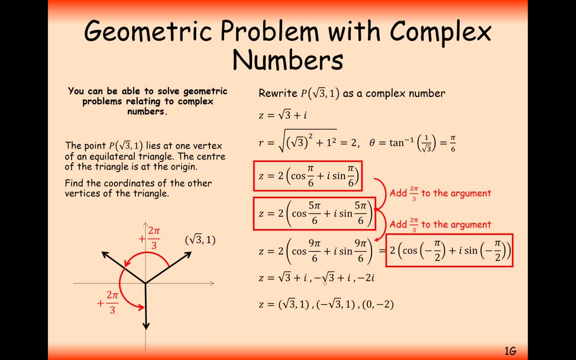 the complex numbers as coordinates. So root 3 plus i minus root 3 plus i and minus 2i. So there we have it. That's the answer to this question. We've found the other vertices of the equilateral triangle minus. 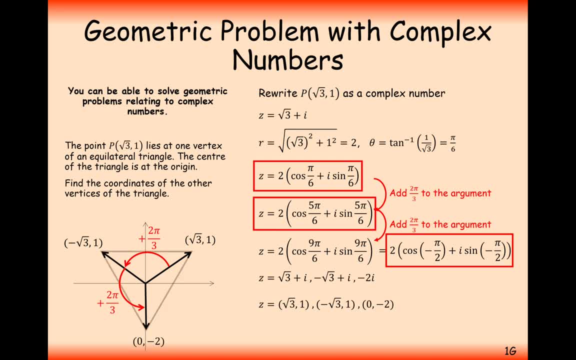 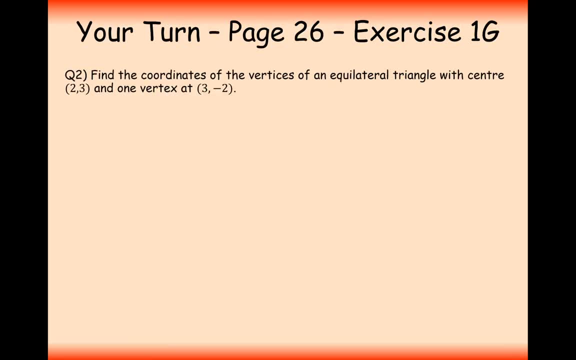 root 3, 1, and 0, minus 2,, making ourselves a perfect equilateral triangle there. Let's move on to question 2 of exercise 1g. a little bit of a challenging problem. That's why I've given it, so I've put it in this video. So pause the video and give this question. 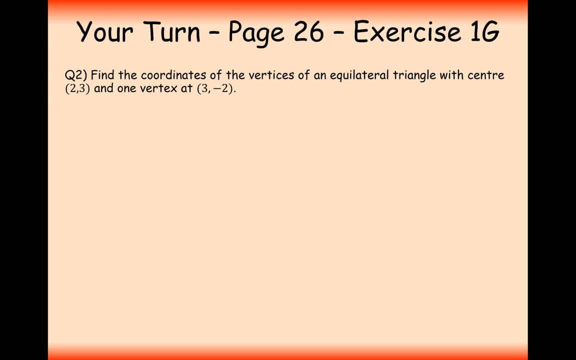 a go. Okay, so let's have a go at this question here now. Now it's a different question to the one we've just answered, because this question says: find the coordinates of the vertices of an equilateral triangle with centre 2, 3.. So that's 2, 3.. So centre here, and 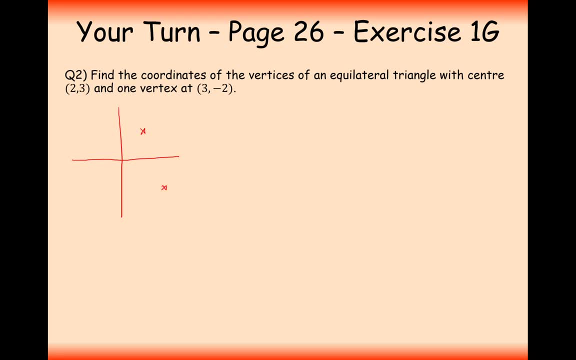 vertex 3, minus 2.. So that's down here Now. what we're going to need to do first is work out the vector from the centre. So that's down here Now. what we're going to need to do first is work out the vector from the centre to the vertex and then rotate that. 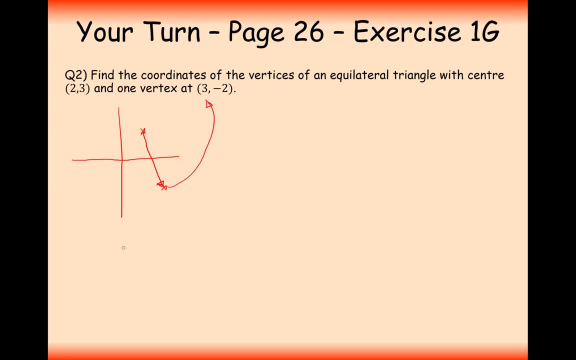 around the centre by 2, pi by 3.. So what I'm going to do is I'm going to transform this question into having a centre 0, 0, and then this vector is going to be right by 1, down by 5.. So right by 1,, down by 5.. So it's actually going to be at a coordinate: 1, minus 5, down. 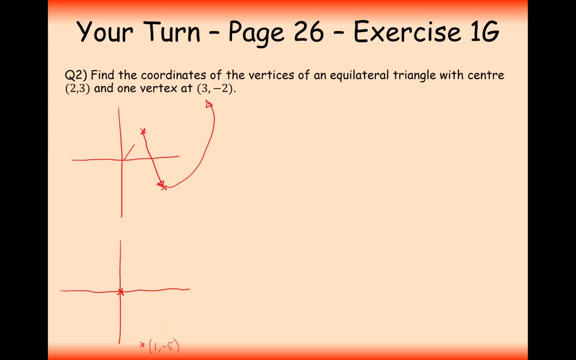 here And I'll rotate this around the circle and then I'll just add 2 plus 3i onto my first and final answers. So here we go. We're going to take 1, minus 5i and first work out the 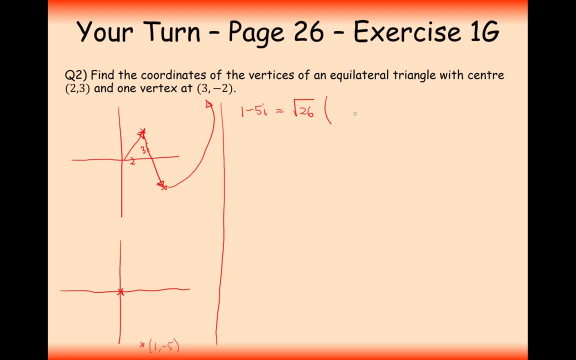 modulus, which will be root 26.. And the argument here: let's just do tan inverse. It's going to be minus cos minus 1.37, plus i sine minus 1.37.. So the first argument we're going to: 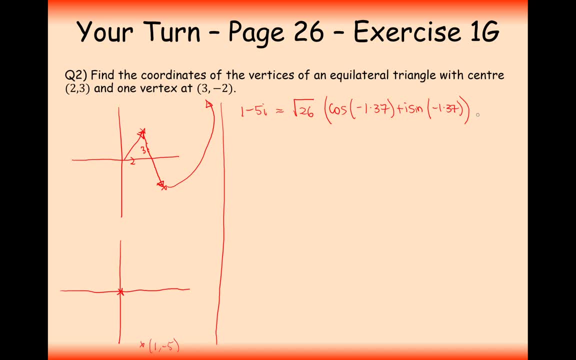 use is tan inverse. It's going to be cos minus 1.37 plus i sine minus 1.37.. So we would 0.37.. And now we'll just add 2 pi by 3 onto the argument. So the next answer is going. 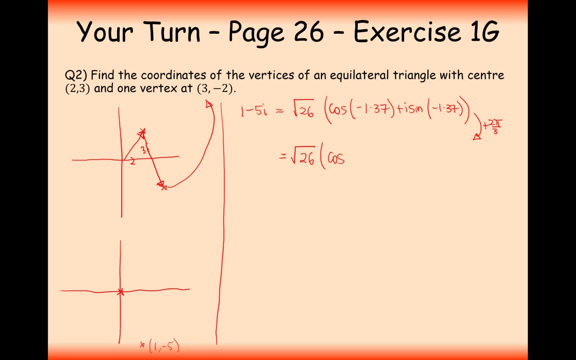 to be cos and add 2 pi by 3.. So the next one is going to be 0.72 plus i sine 0.72.. And then we'll add 2 pi by 3 round again, and that will give us: 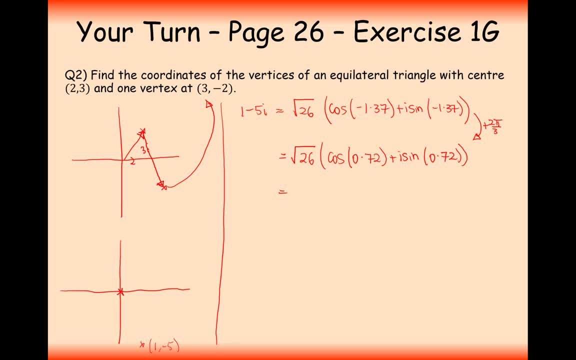 0.72.. So let's just work that out: 2.82.. So root 26, bracket cos 2.82, plus i sine 2.82.. Okay, Okay, Okay, Okay. So those are the relative positions when we just add around 2.8.. So 2 pi by 3. 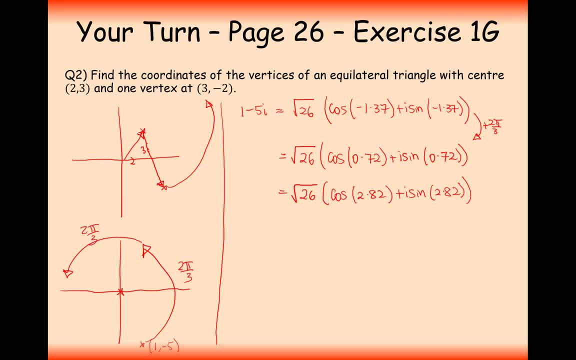 around the circle. So now we've got to find the vertex from the relative position of 2 plus 3i. Well, the first thing we'll do then is we'll rewrite out both of these as complex numbers. So let's expand the brackets on the modulus argument form, And the first one's. 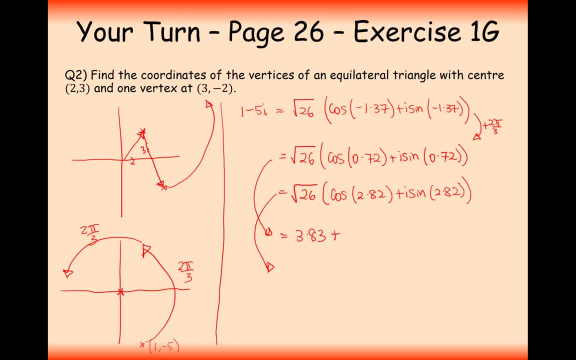 going to be 3.83.. Okay, 3.83 plus 3.63i. And the second one is going to be minus 4.84 plus 1.61i. Okay, So now what I've got to do is I've now got to add 2 plus 3i. 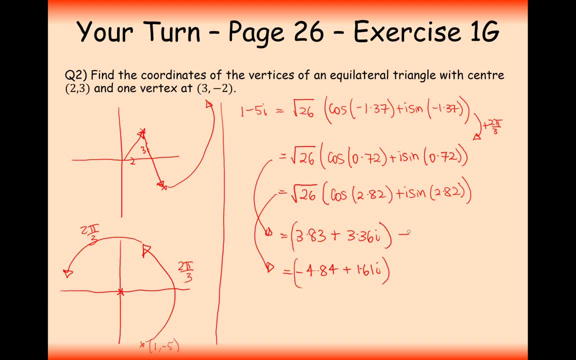 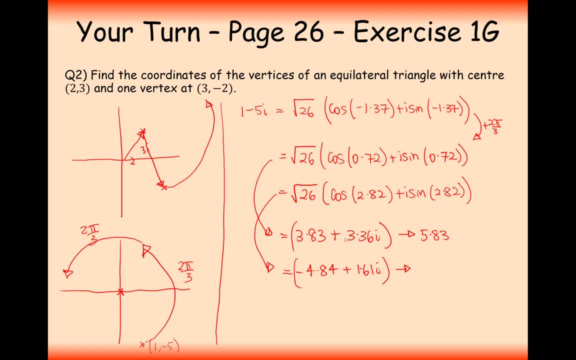 Okay, Okay, Okay, Okay, Okay Okay. you can see I've got toως all of those a little times because many of our cases and the ones that… I'm really bad at these things, but all my units of Episode 15 started out to be about.